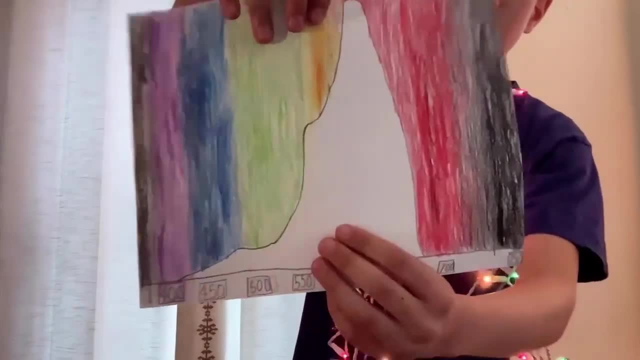 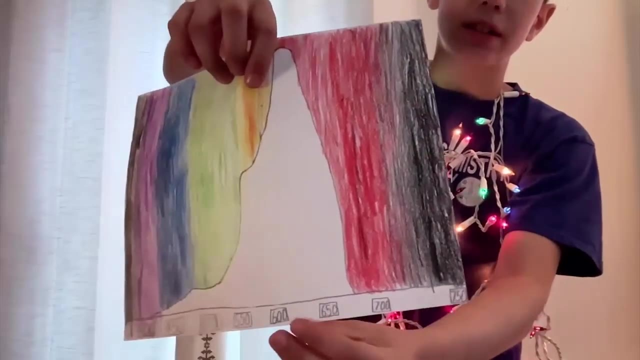 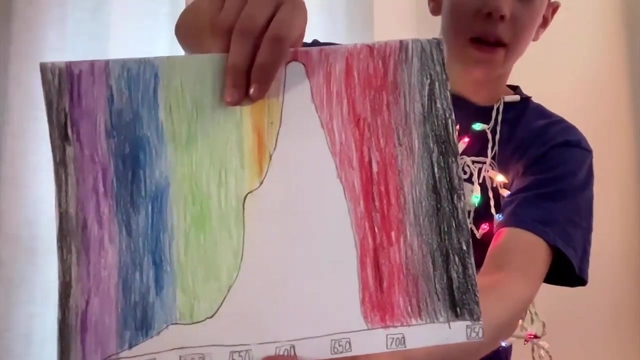 and the absorbance spectrum for thalassinide would look something like this: These colored pigments absorb the opposite wavelength light- a yellow, orange and red. that is roughly a 600 to 650 nanometer wavelength, and emit a lower 450 to 500 nanometer light, which 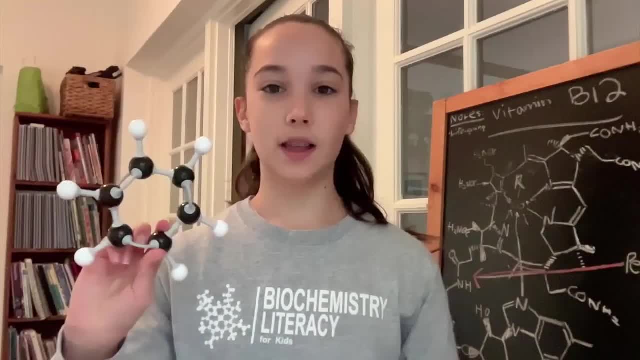 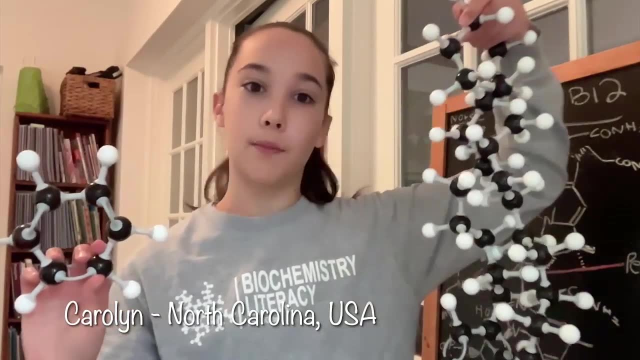 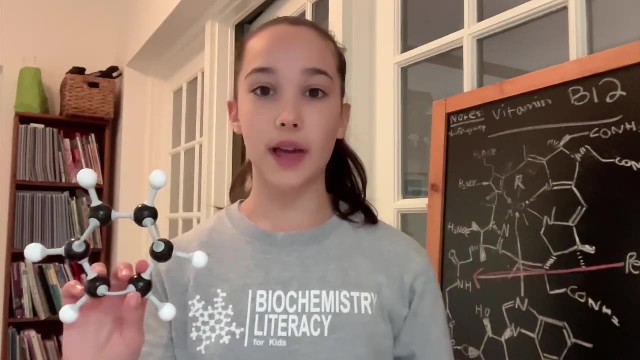 is blue. Something else Dr Freitas taught us is free radical polymerization. This occurs when a polymer like this example of polyethylene, better known as plastic, forms by continuous addition of free radicals. What are free radicals? These are atoms with one or more unpaired. 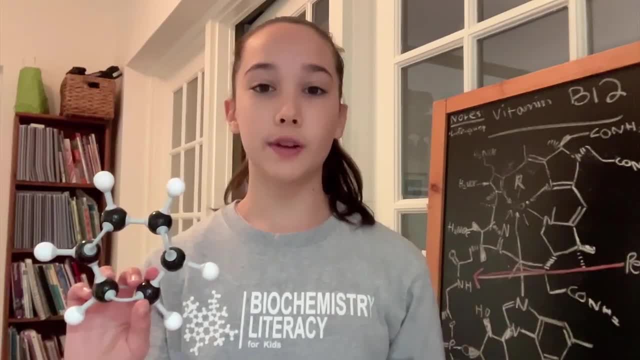 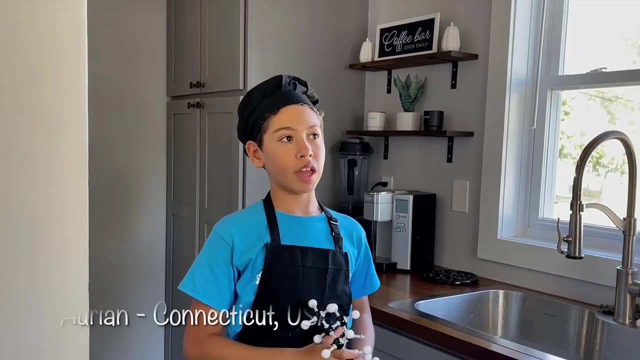 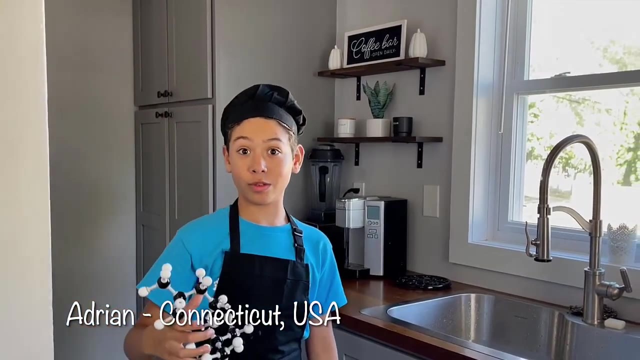 electrons, which makes them very reactive. These free radicals add monomer units and the polymer chain grows. Hmm, I wonder if I can make lemonade with this limonene molecule, which is also found in lemons. Only one way to find out: I need to squeeze harder. Look, it's working, It's. 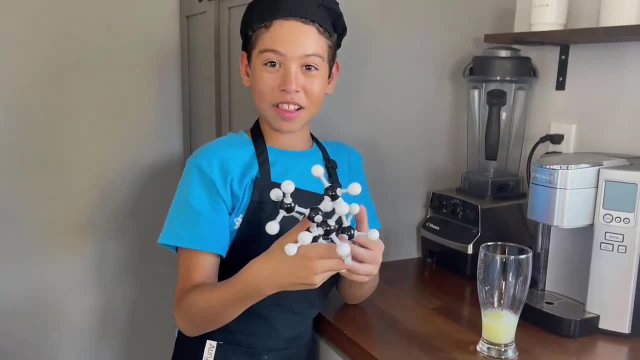 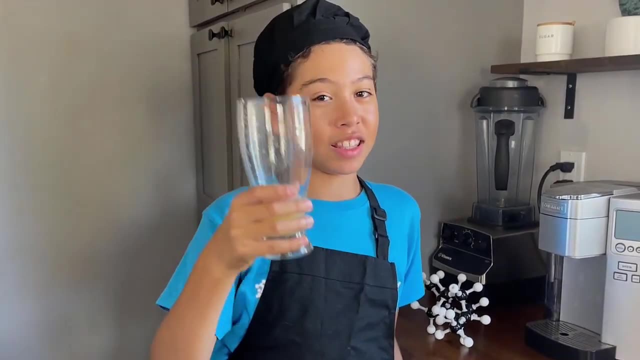 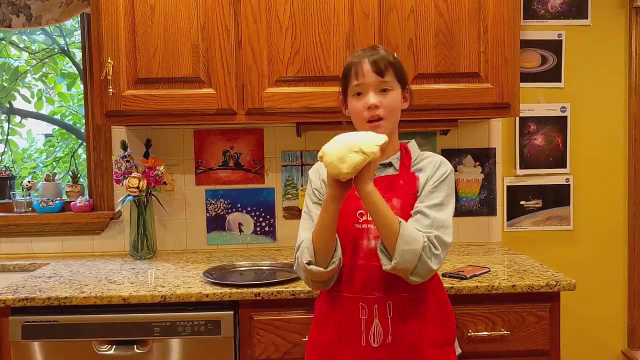 working. Thank you, molecule. Now let's taste this 1.8% of limonene inside this lemonade Sour, Oh hi. Would you like to know what makes dough rise? Well, it's all because of yeast. 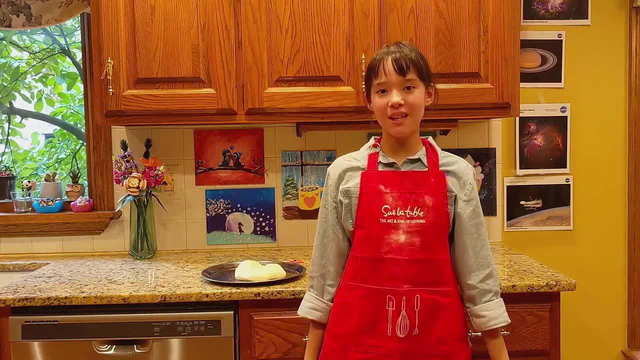 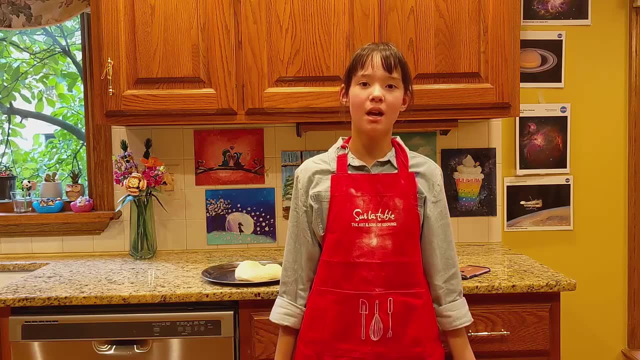 Yeast performs something called a fermentation reaction. A fermentation reaction is a reaction in which an organism is deprived of oxygen and is forced to find other ways to metabolize. It produces carbon dioxide, which causes the dough to rise. I learned a lot of science. 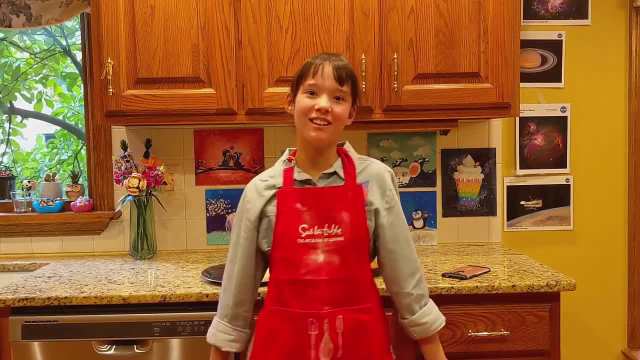 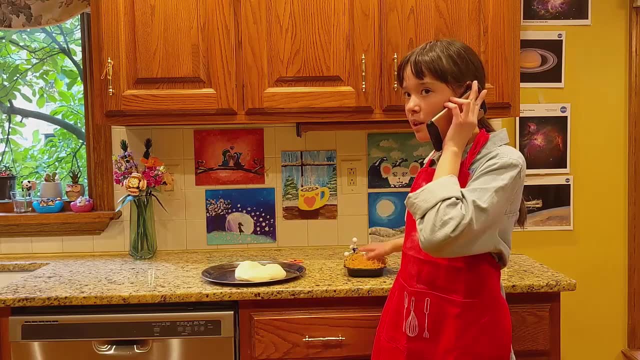 from Dr Freitas' class, and if you go to summer camp, you can too. Give me a moment. I need to take this order. Chubbell Right, Chubbell Sure Pizzeria. One more pizza coming up. 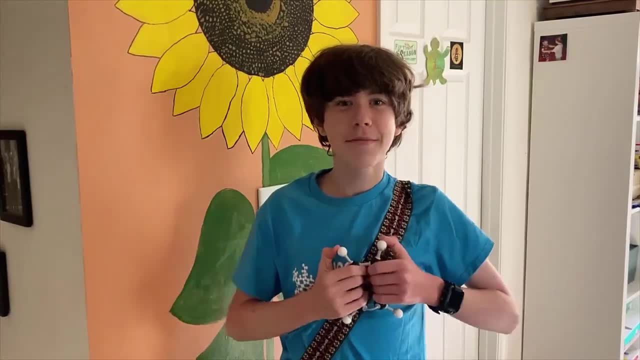 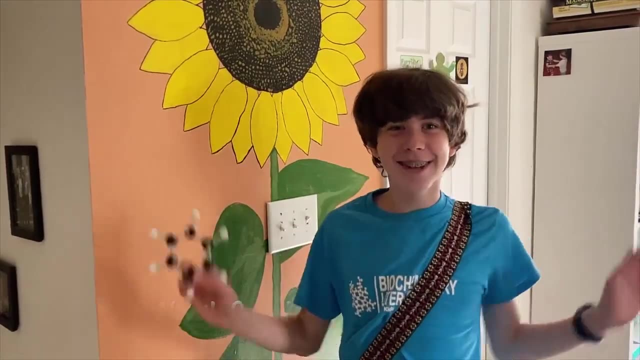 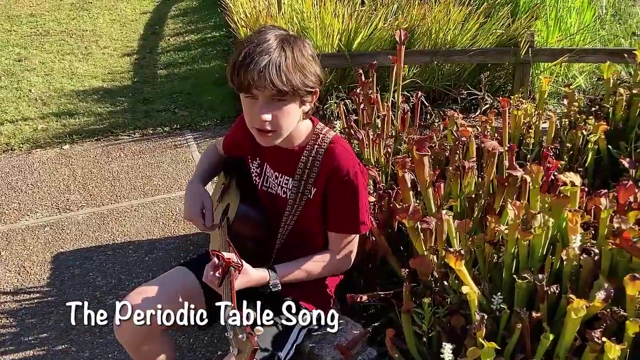 Mozzarella, Pepperoni. Five-pounds of carbon. Dr Freitas' program has gotten me so interested in the periodic table that I can't stop singing about it. There's hydrogen and helium, One, two, three, four billion, five, four billion. 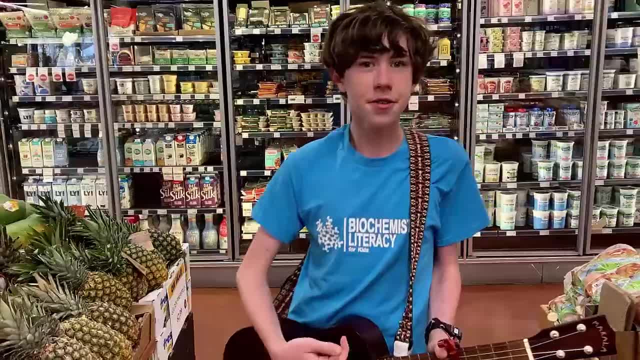 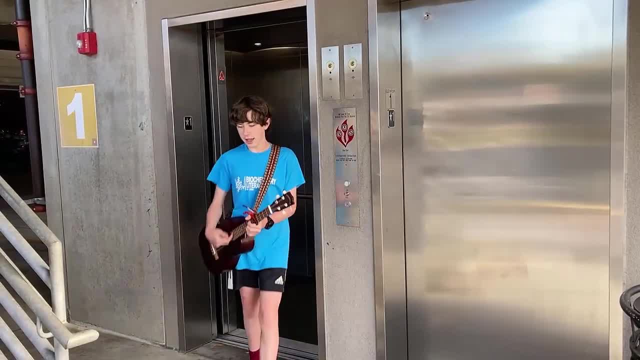 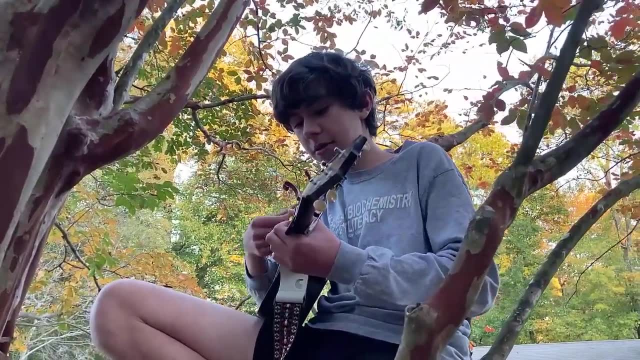 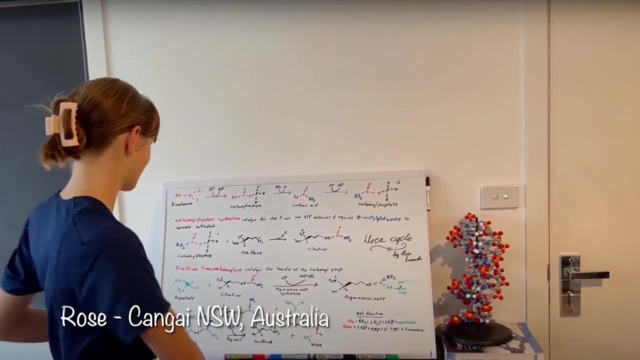 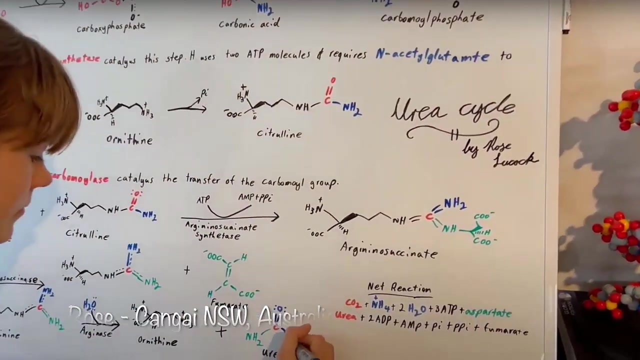 One, two, three, four million. One, two, three, four billion. One, two, three, four billion. Hi, I'm Rose. Urea can cause kidney failure if it is produced in large amounts. They call this uremia. Uremia is caused by a buildup of toxins in your blood and most likely lead. 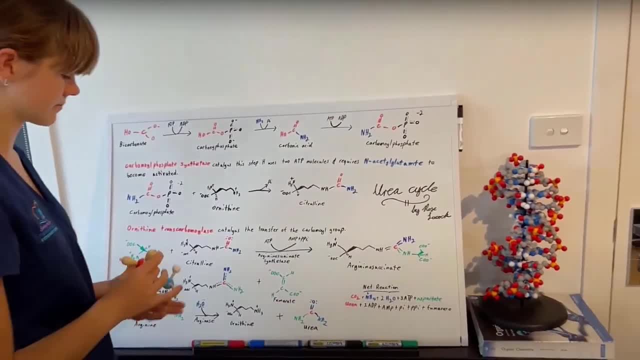 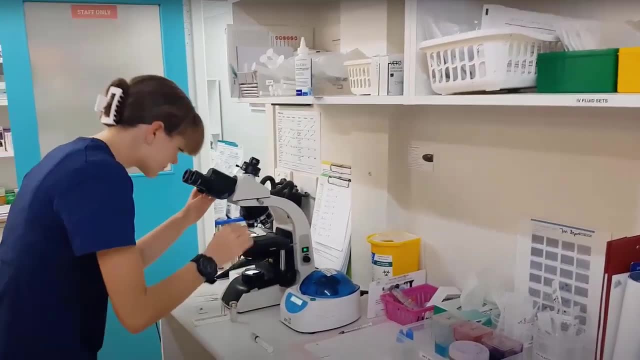 to kidney disease. The kidneys go through this mechanism, as you can see on the board making urea, for it is a major source of being filtered through the kidneys. removing the other waste products from the blood In animals, we use the terms excretion of nitrogenous. 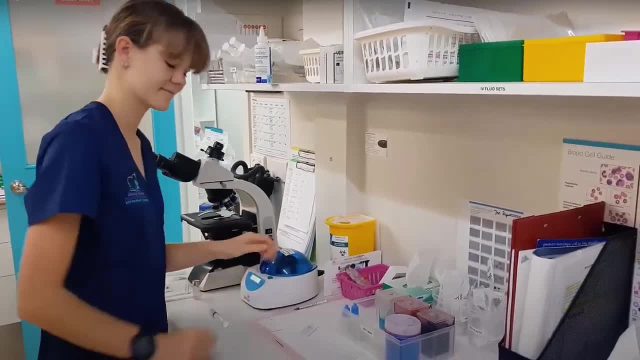 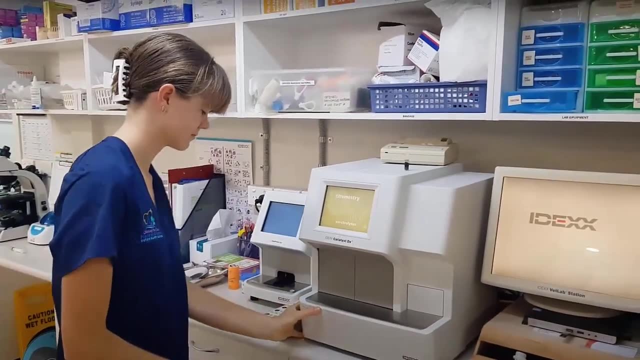 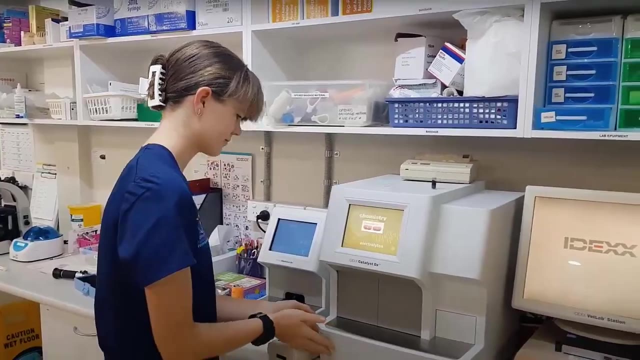 waste Testing for uremia. in the kidneys we use a bum blood test. Even in animals we use a bum blood test to test for high levels of urea. Dr Fried has given me so much knowledge in biochemistry and I can use this knowledge in my work at my local veterinarian hospital. 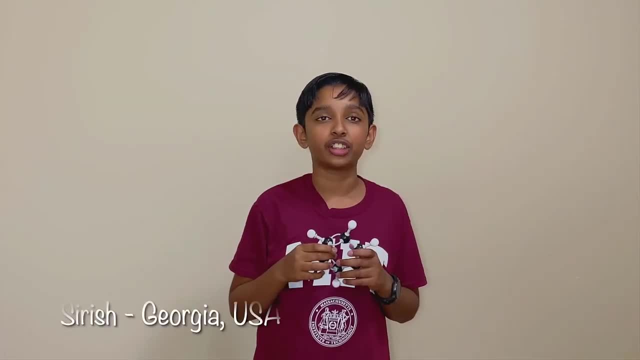 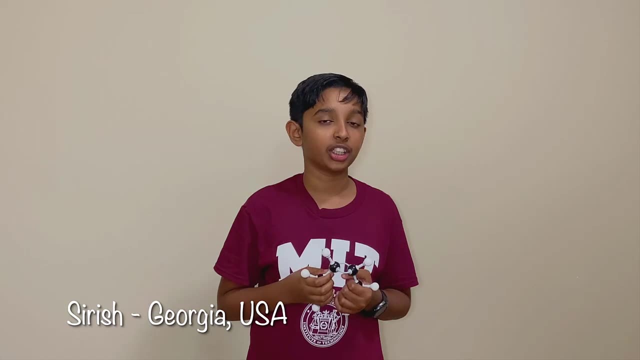 Biochemistry is essential for understanding how medicines treat disease. One example is targeted cancer therapies. Monoclonal antibodies, or MABs, are designed under the principles that Dr Fried has taught us. In our online classes, we have learned about hydrogen bonding. 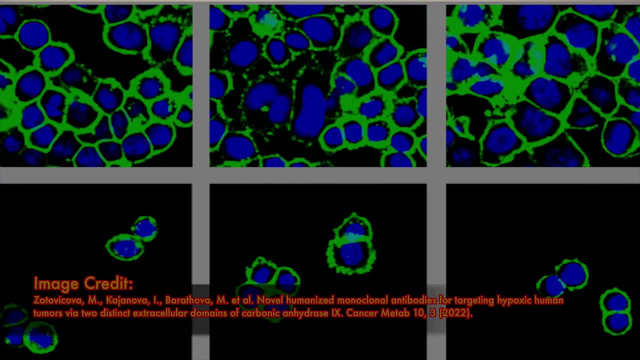 which is important to designing the receptors, or MABs. When arranged correctly, these receptors can bind to cancer cells and flag them, For example, if you have a cancer cell, you can use these receptors to bind to cancer cells and flag them, For example, if you have a. 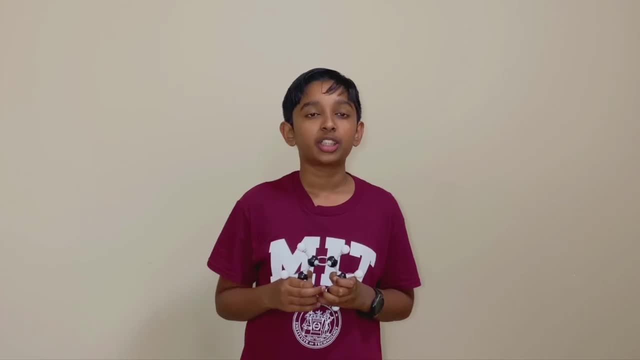 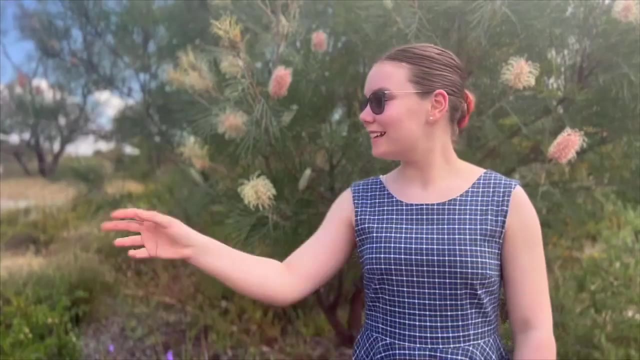 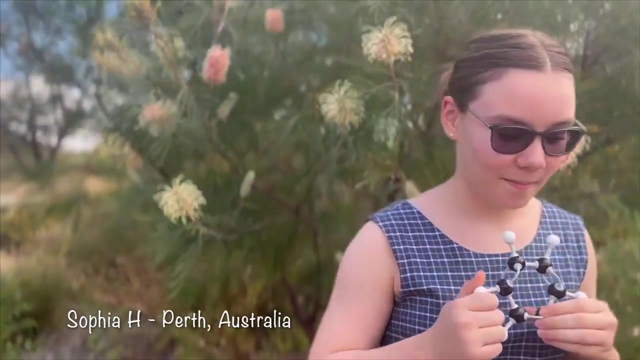 cancer cell. you can use these receptors to bind to cancer cells and flag them. For example, if you have a cancer cell, you can use these receptors to bind to cancer cells and flag them. At summer camp we'll be learning the lab authorities' effective. 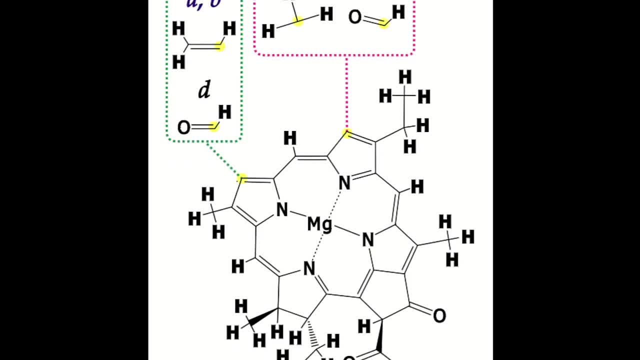 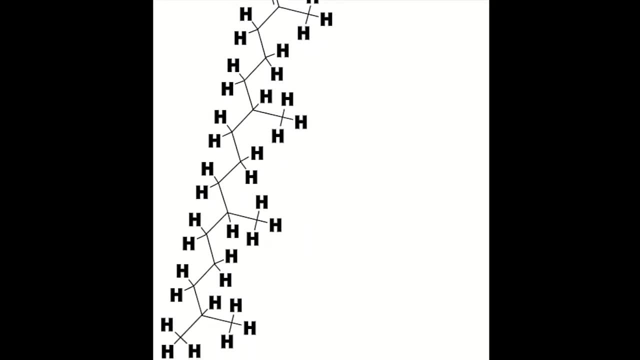 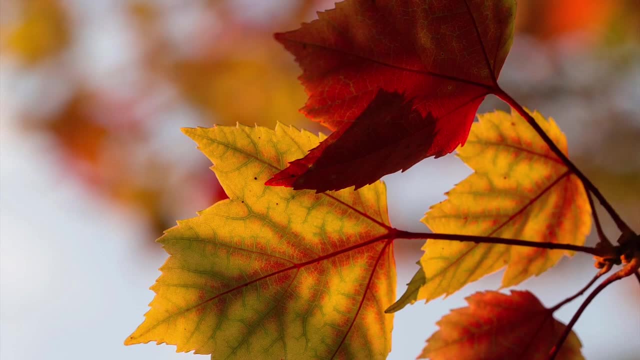 致 Unit感染結果. This lab supercomputer actually needs to work in advance for now, and so we'll send off our doc staff지� Bi Tacta. Hi, I'm Seop, I'm Doctor. and oceans to trees such as the grevillea. you can see now Chlorophyll is. 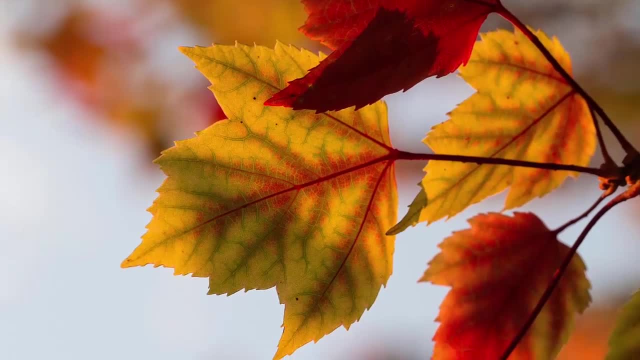 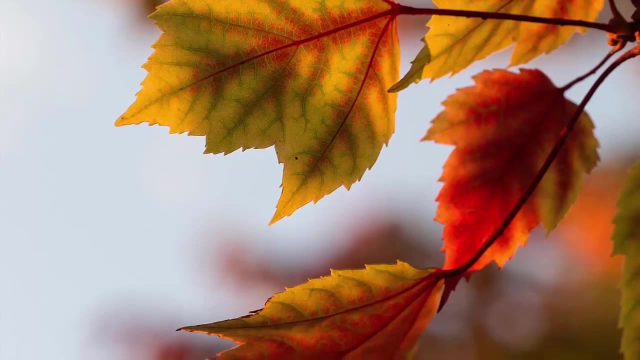 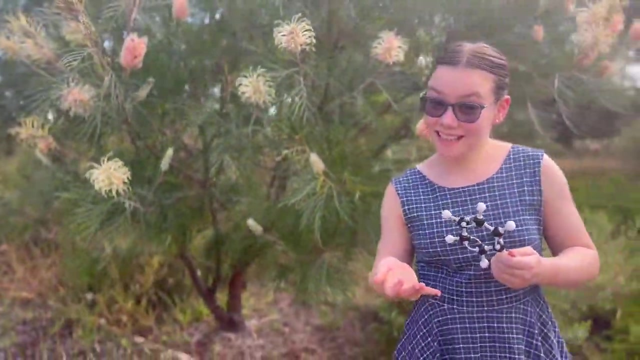 vital to plant photosynthesis and can disappear inside a tree and fall, which is what makes the leaves of the tree turn brown. Obviously, this doesn't happen in all trees, which is why we have evergreens, so biochemistry really is everywhere. Do you see what I mean? 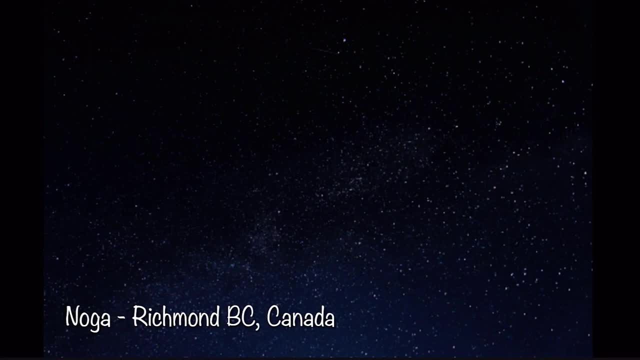 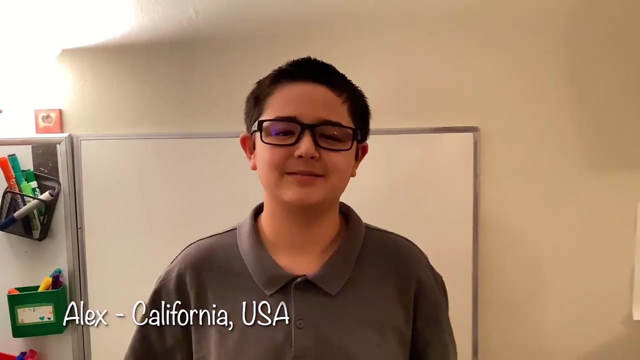 Did you know that stars are the factories for new atoms? and since you're made of atoms, you're made of stardust, so anything that has mass is made from a star, like all the planets. Star chemistry is truly wonderful. Hello, I'm Alex, and me and everyone here in Biochemistry, Larry Sivakas classes. 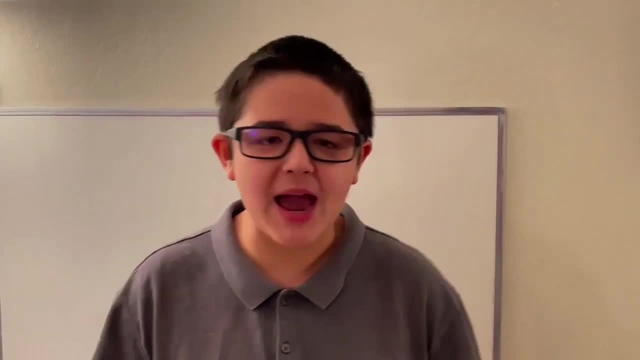 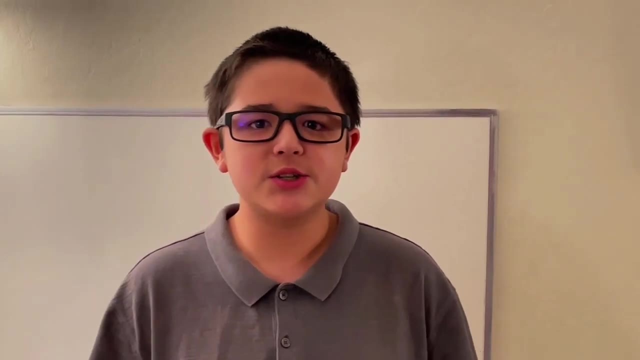 We love science. It is our life. This is our passion. This is what we're gonna do with our life. We're gonna teach our children science, and science is what we're gonna do when we grow up. This camp will help us do experiments that people don't get to. 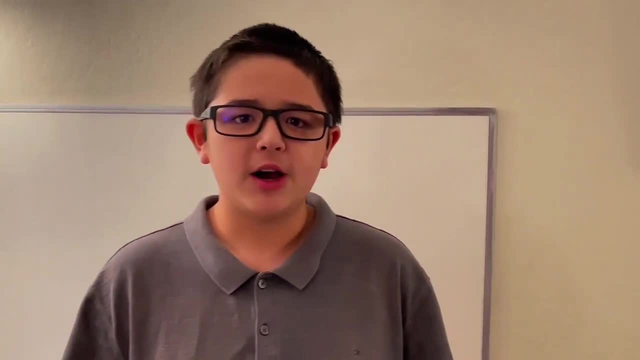 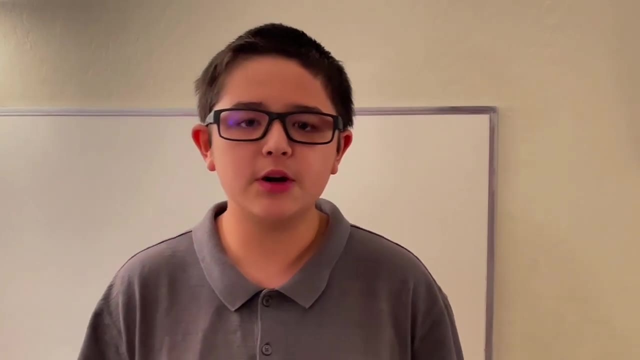 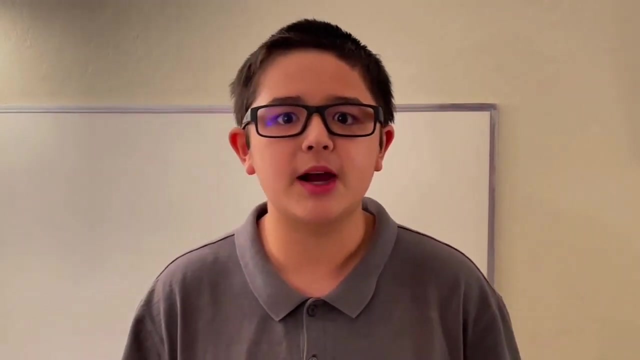 do until they get into college. This camp will help us apply our knowledge to the real world and do experiments like PCR testing, protein expression and protein extraction. Dr Fried has already proven that kids in elementary and middle school can do organic chemistry and biochemistry. With your sponsorship, this camp will put 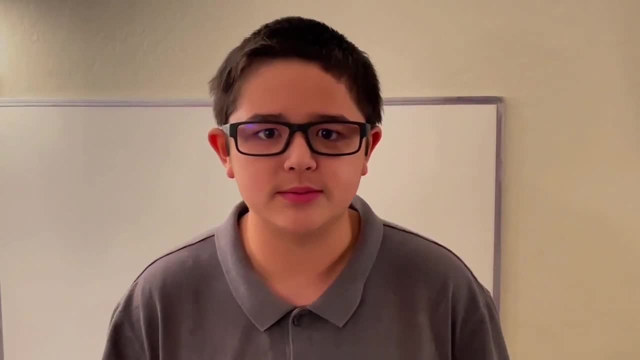 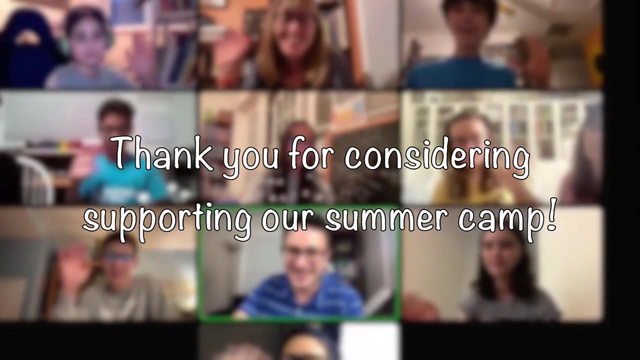 us on accelerated courses and help us to solve tomorrow's problems. On behalf of all of us, thank you for considering supporting our summer camp. Hi, I'm Dan Fried and I'm the creator of Biochemistry Literacy. If you are interested in, 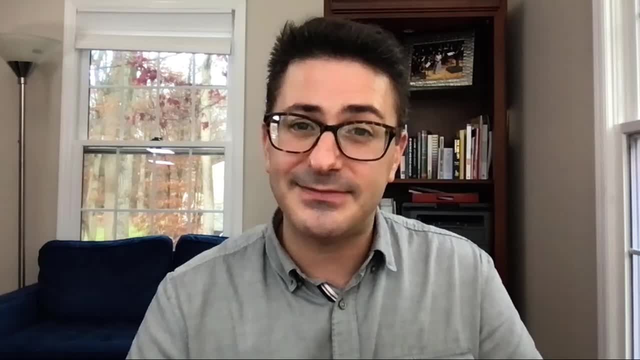 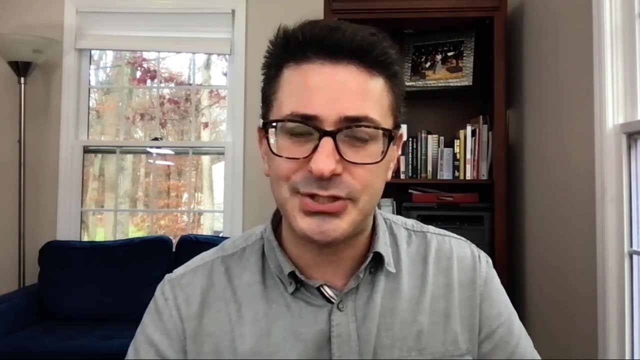 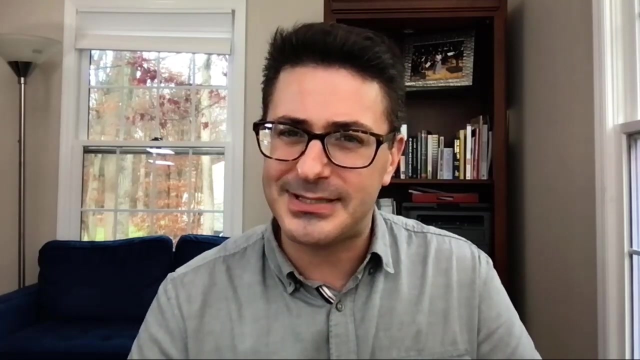 learning more about the program or the upcoming summer camp, please visit the project website biochemistryliteracyforkidscom. I began working on this program around 2011 as a PhD student at Yale University and over the years, it has really grown into something amazing and really unprecedented. You can see what. 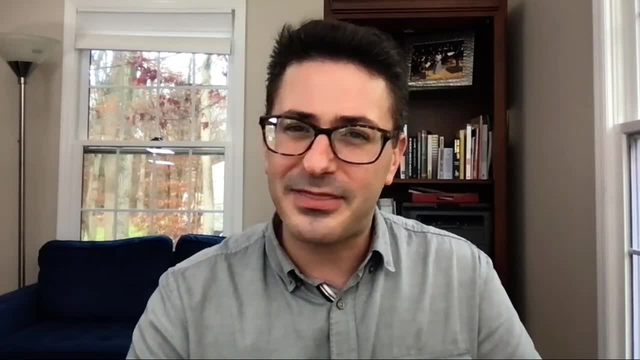 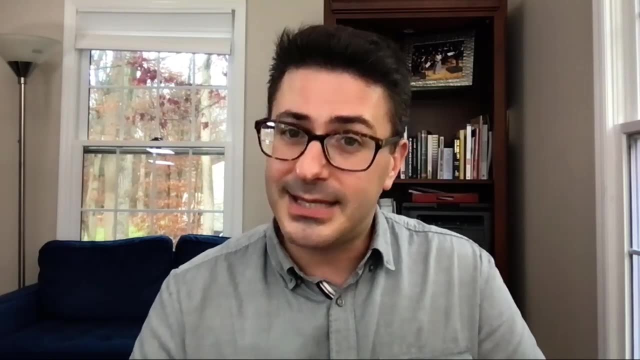 an effect it has on these kids' lives. Right now, there are around a thousand homeschool families that have used the program, as well as many, many students in public and private schools- The kids that you just heard from. they really want to bring more of their friends to this camp in Pottersville, New Jersey, and there's 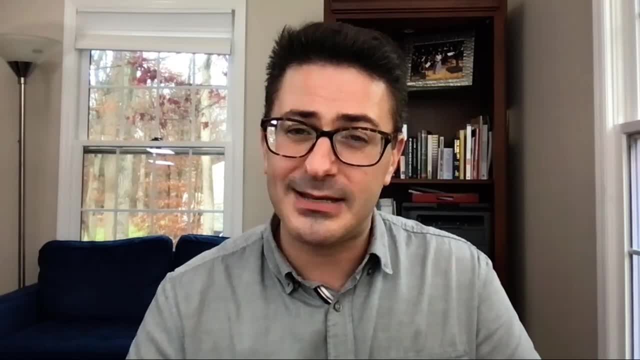 ways to make that possible. If you want to help contribute to this, you can navigate through the website to the contact page and you can make a donation through Patreoncom. You can post your questions in the post and I want you to through the PayPal link there.